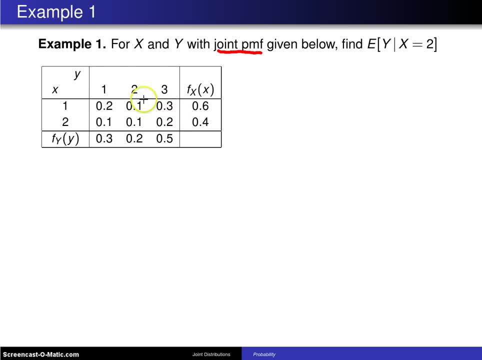 Well, here is the joint distribution and it's given in table form and you'll notice that these six values right here are the joint probability mass function. and when we're looking at x equals 2 as the given part of that expression, you know automatically that you are down in this area. 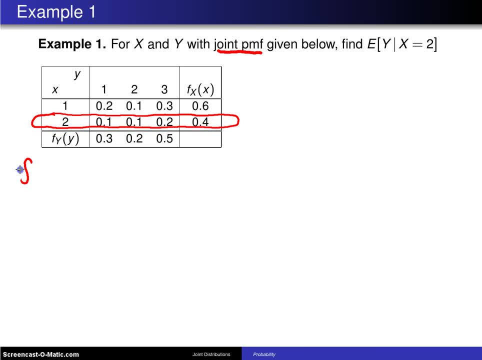 right here. So the first step to finding this conditional expected value is: we have to find the conditional probability mass function of y, given that the random variable x is equal to 2.. Now, in this particular case, we will have three different values for y, that is, 1,, 2, and 3.. So we'll put these out over here. 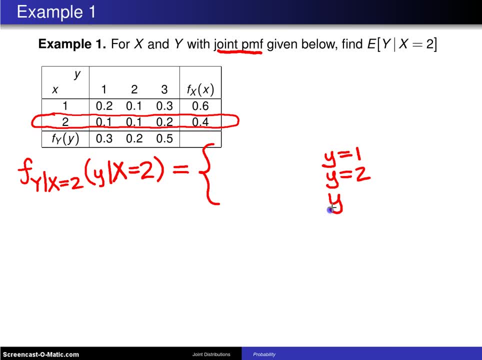 as the support. and if you remember the definition of a conditional distribution, it is the ratio of the joint pdf to the marginal. So, for the case of y equals 1, you will get 0.1 divided by 0.4, which is one-fourth, and for y equals 2, you will get 0.1 divided by 0.4, which is also one-fourth. 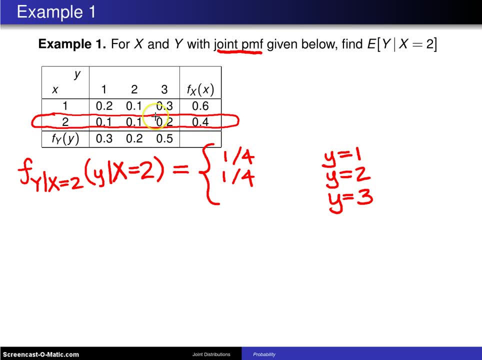 and then for y equals 3, you will get 0.2 divided by 0.4, which is one-half. These three values sum to one, so we have a legitimate probability mass function. Now the next step to find the expected value of y, given x is equal to 2. 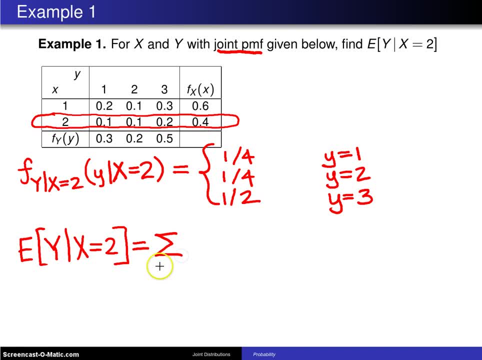 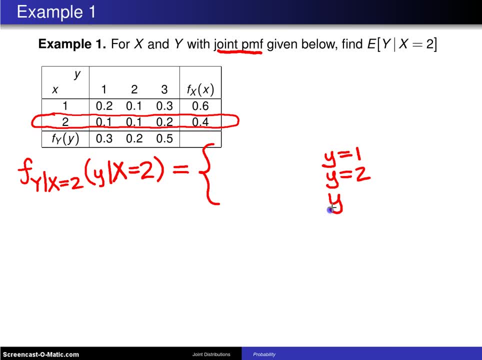 as the support. and if you remember the definition of a conditional distribution, it is the ratio of the joint pdf to the marginal. So, for the case of y equals 1, you will get 0.1 divided by 0.4, which is one-fourth, and for y equals 2, you will get 0.1 divided by 0.4, which is also one-fourth. 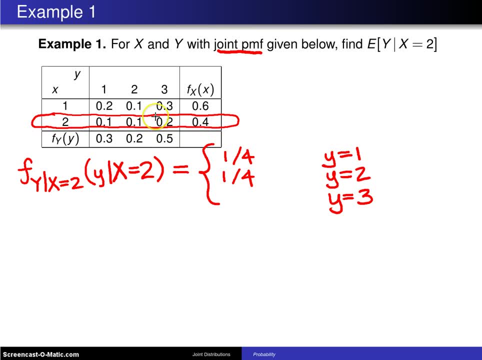 and then for y equals 3, you will get 0.2 divided by 0.4, which is one-half. These three values sum to 1, so we have a legitimate probability mass function. Now the next step to find the expected value of y, given x is equal to tre. 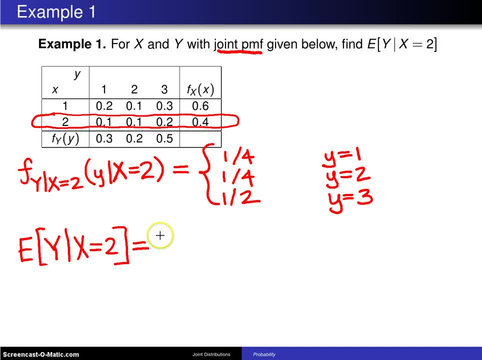 To 2.. By definition, that will be the sum Overall Y, and in this case Y, runs from 1. Up to 3.. Of what we had before was gj of y, will Gif y. y in this case is just y multiplied by the joint- I'm sorry, the conditional probability mass. 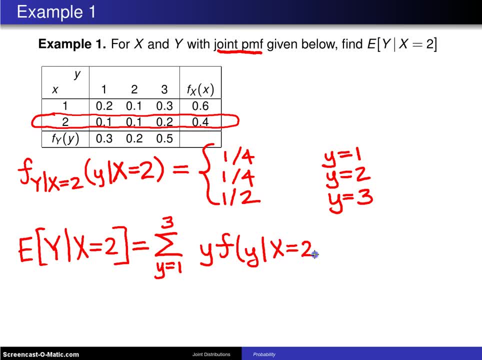 function f of y, given x is equal to 2.. So in this case we get 1, which is right here- multiplied by 1 fourth plus 2, multiplied by 1 fourth plus 3, multiplied by 1 half. and when you work that out, 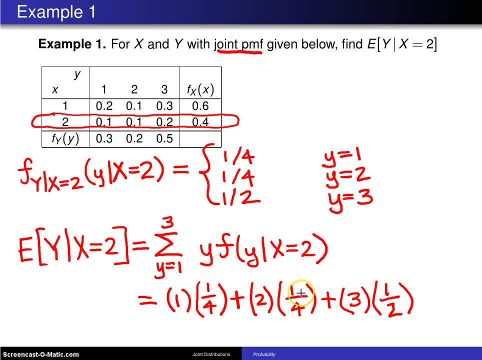 that's going to be 1 fourth plus 2 fourths plus 6 fourths and that turns out to be 0. 9 fourths or 2 and a quarter.